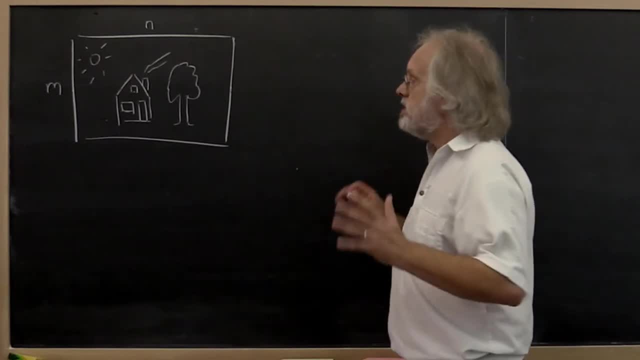 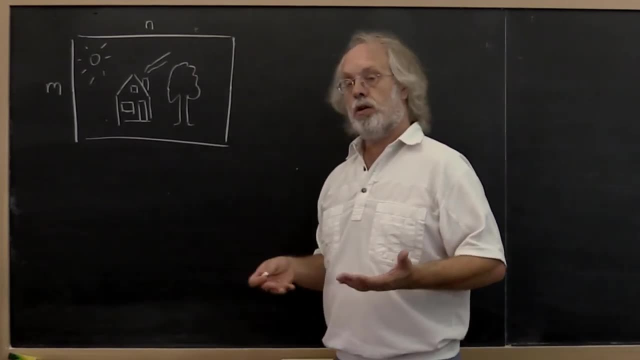 But we're going to motivate it by looking at a picture. So what's the idea? Well, let's say you take a picture with your digital camera. The picture really is stored as a two-dimensional array of pixels, And pixels really are numerical. 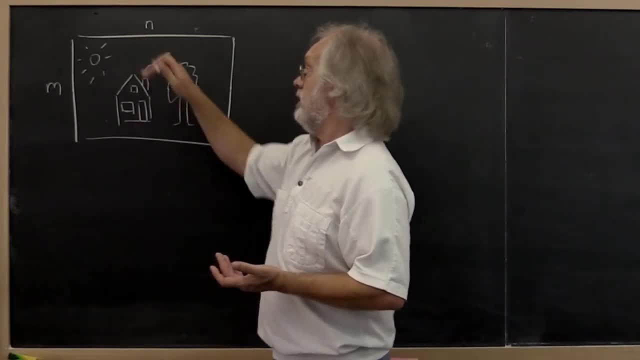 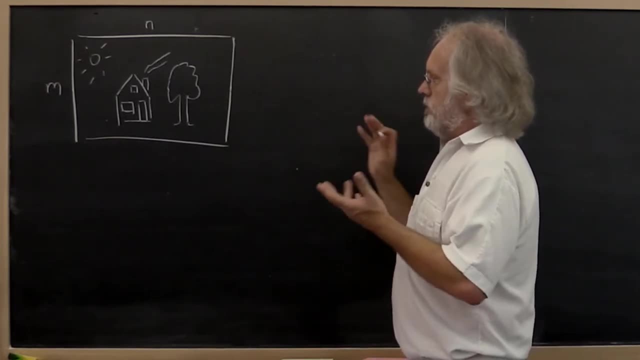 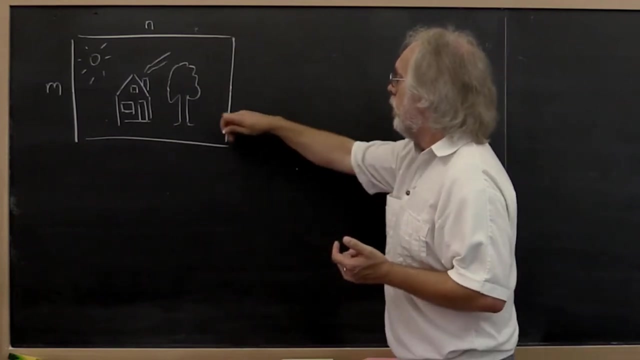 values. So we can think of it as an n by n matrix. Okay, so what if we don't want to store all of the pixels? What if we want to somehow do data compression? Well, if we call this the matrix B, then what we may want to do, 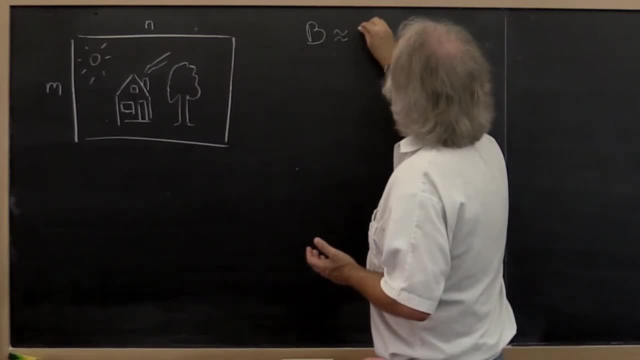 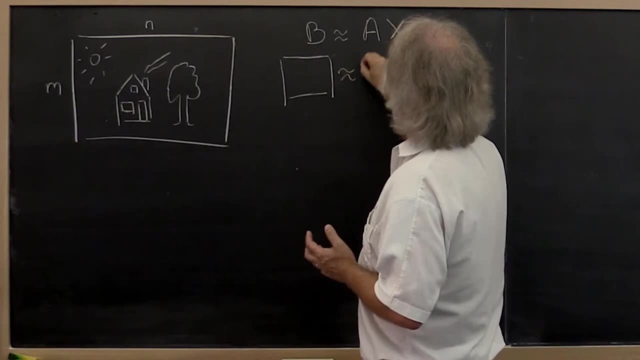 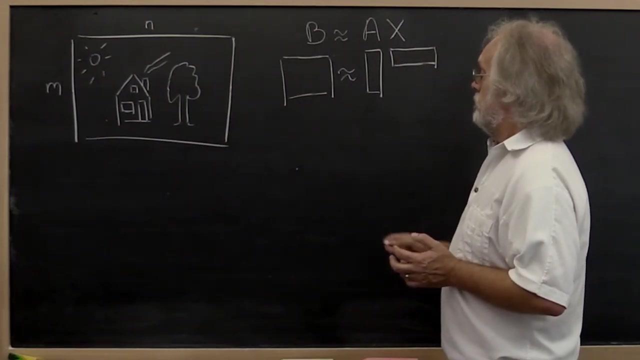 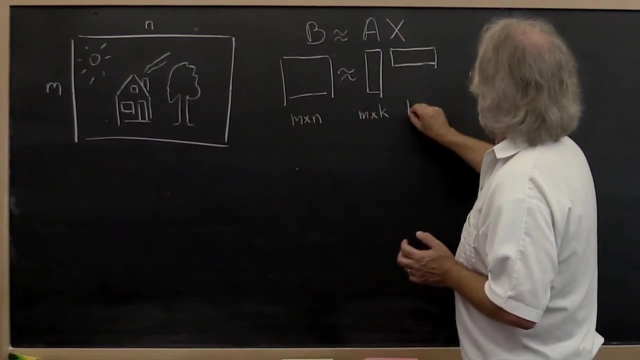 is approximate this with a matrix A times a matrix X, where the idea is that matrix B is the entire picture. A is a matrix with only a few columns and X is a matrix with only a few columns. B is n by n, A is n by k and X is k by n. 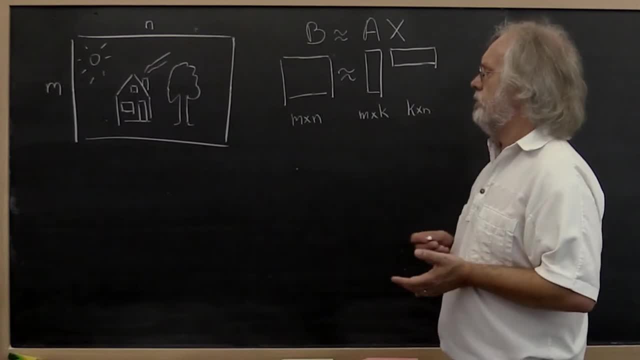 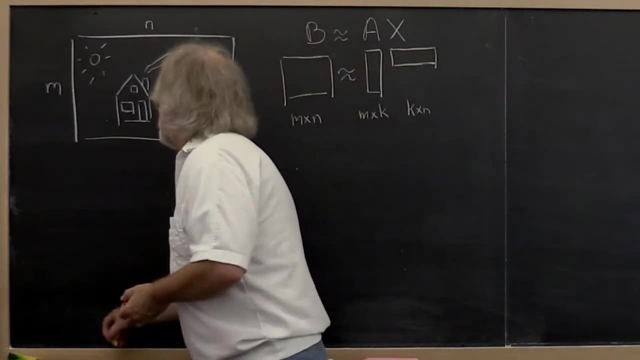 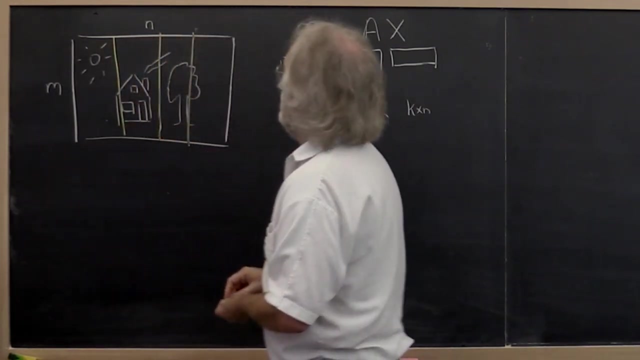 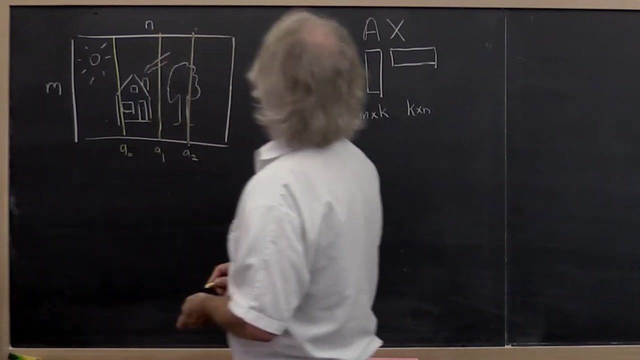 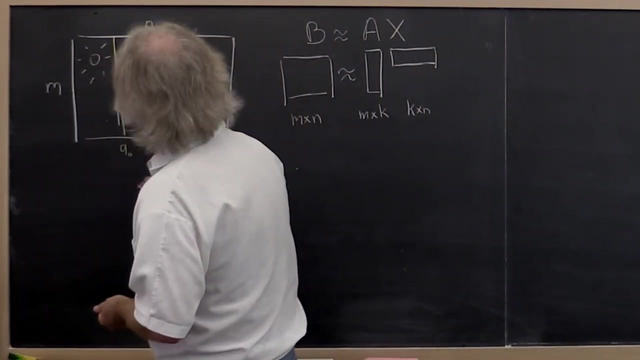 Alright. Well, how might we do this? Well, one way for coming up with matrix A could be to say: okay, we'll pick a couple of columns in our picture and we'll make those the columns in our matrix A, Alright. And then, if we take an arbitrary column in 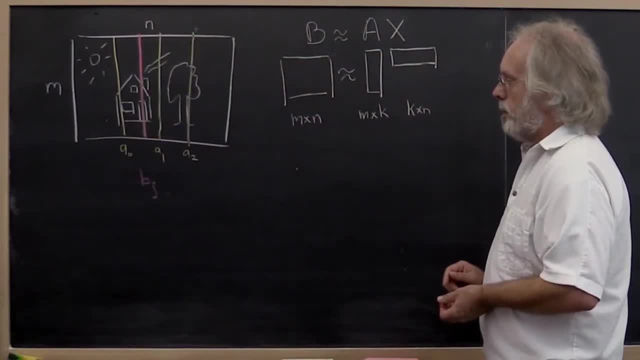 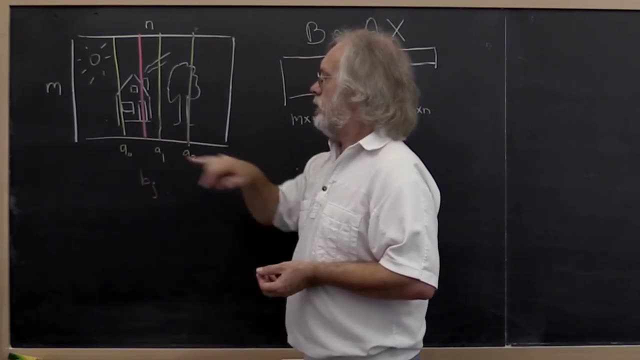 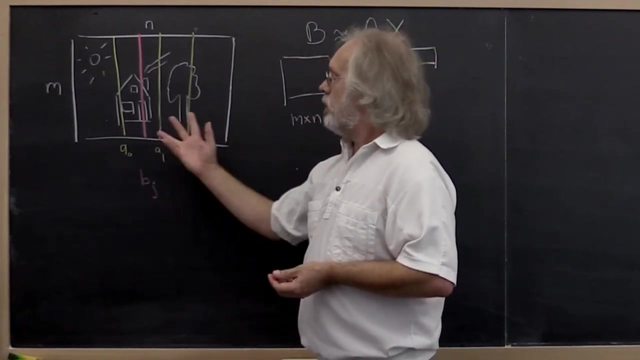 our original picture. let's call it Bj. we're going to say, hmm, if the columns that we picked represent the picture, then maybe we can approximate this column Bj as a, as a linear combination of the columns that we picked for A. What does that mean? 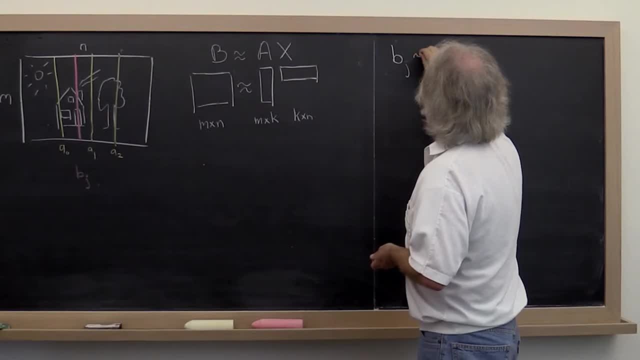 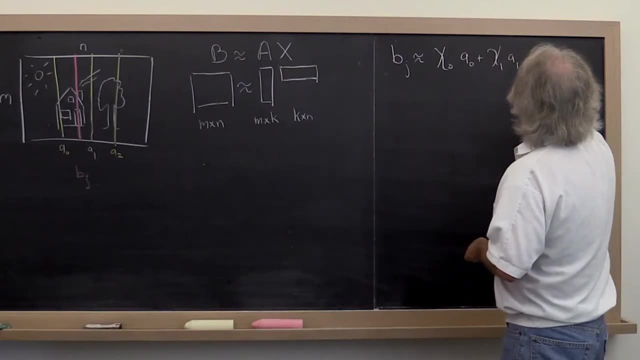 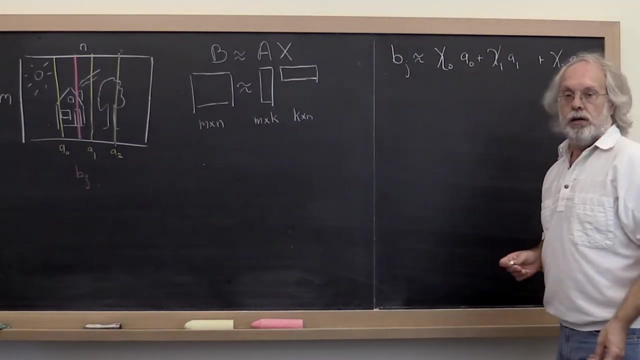 We're saying that maybe B j is approximately some constant chi 0 times A 0 plus chi 1 times A 1 plus chi 2 times A 2. for the case where we pick three columns, Obviously this generalizes to picking k columns. Now we're going to 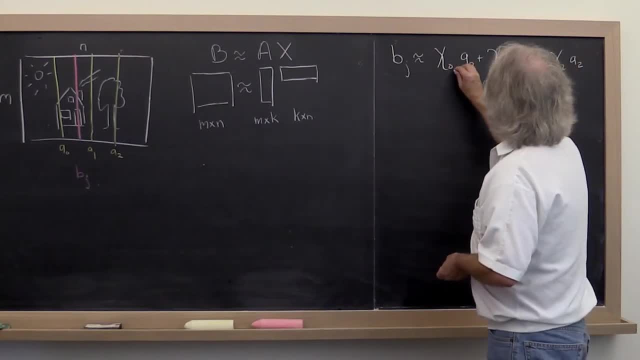 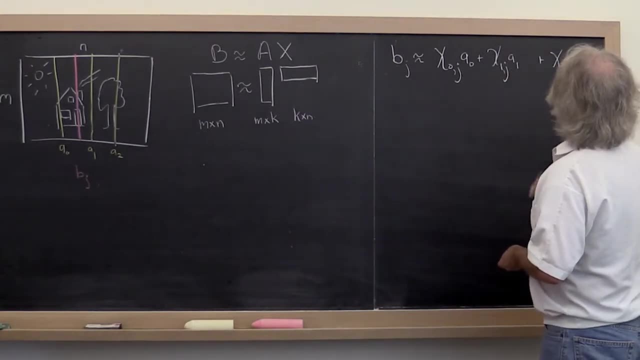 want to do this for every column of B, So we want to bring in a subscript j to indicate that these are the coefficients with which we take linear combinations in order to approximate the jth column of B. All right, Now we said, let's take A: 0,. 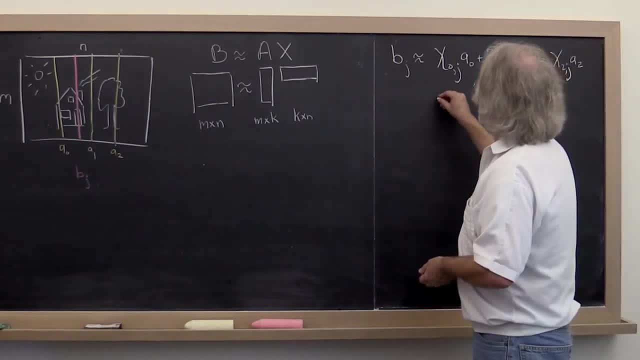 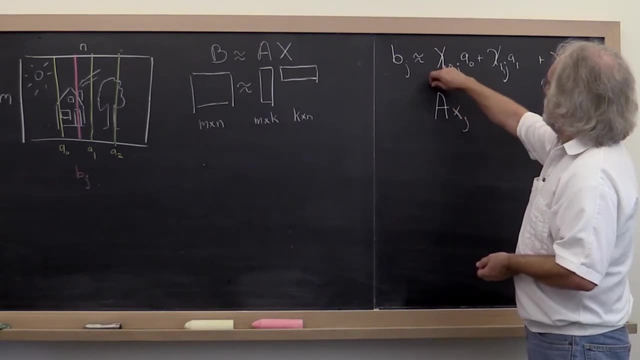 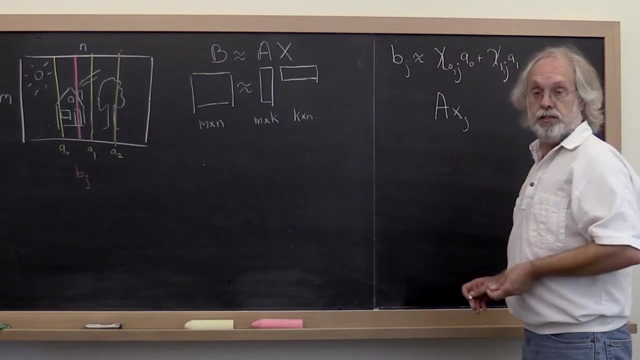 A 1, A 2 to be the columns of A. Okay, So we can also think of this as A times x j, where x j is now the vector, with entries chi 0 j, chi 1 j, chi 2 j or, in more general case, with k entries like that. 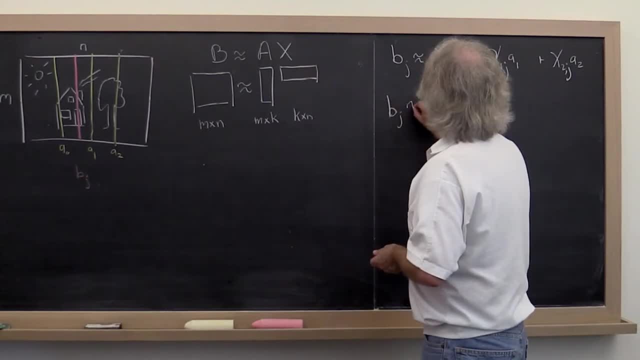 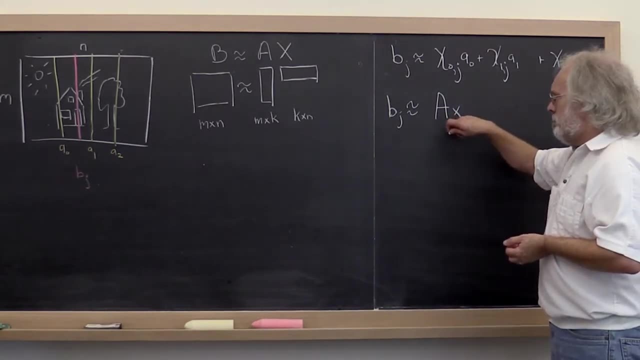 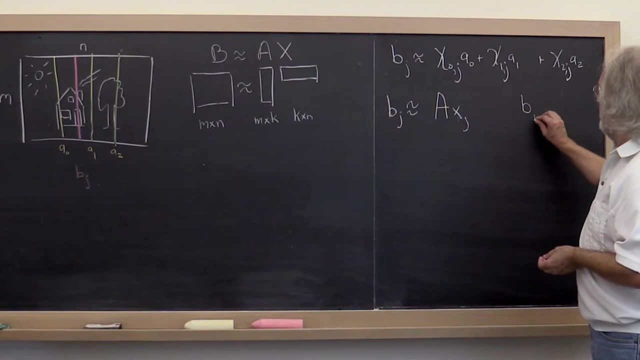 So what we're saying is that B j is approximately A times x j. Now we would like to pick our x j to be the best set of such coefficients. What does that mean? Well, that means that we want to look at B j minus A times x. 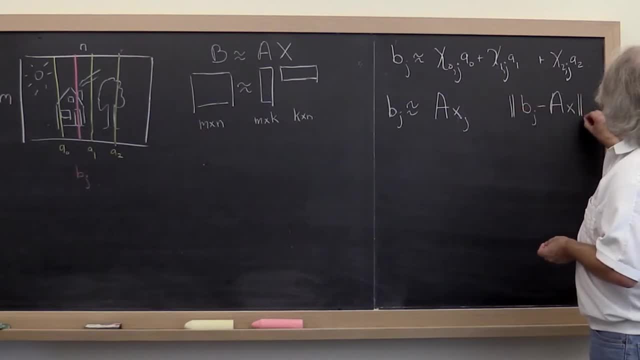 We want to say: let's look at the magnitude of the difference. Well, we can use the two norm for the magnitude And then we can say: minimize that over all possible choices of x and pick your x sub j to be the vector x that minimizes. 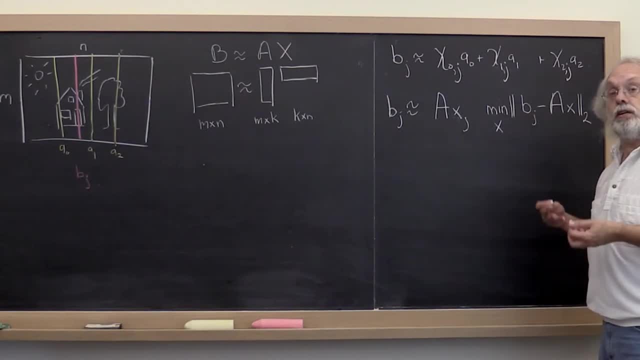 All of that That's known as the linearly squares problem. It's something that you saw in some linear algebra course at some point. It's something we'll delve into much more deeply later. if either you forgot or you didn't see Now, if A 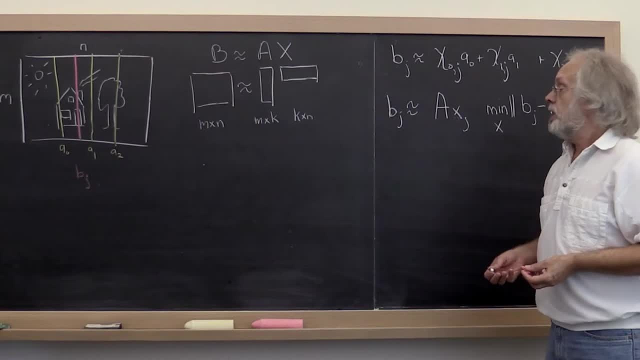 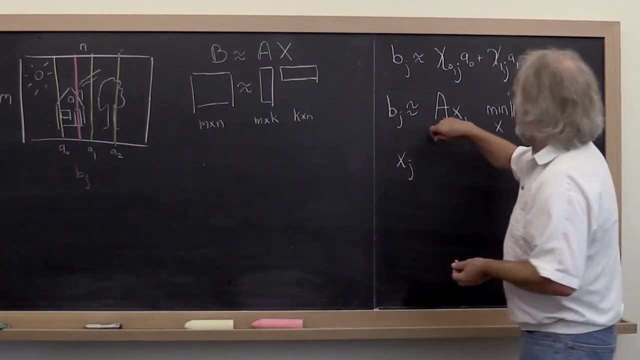 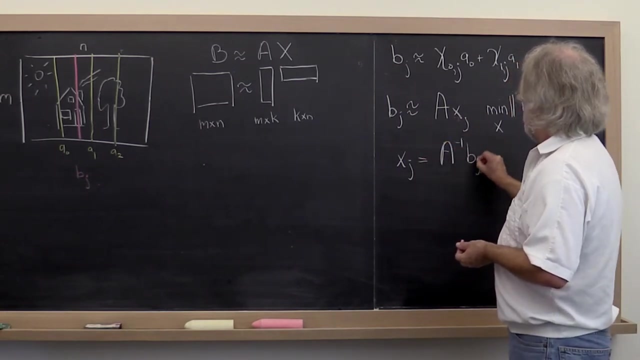 has linearly independent columns, then the best such solution is given by the inverse. Well, let's see: If A were square and invertible, then x- j would simply be A. inverse times B- j. right, But A has more rows than columns in this case. So we 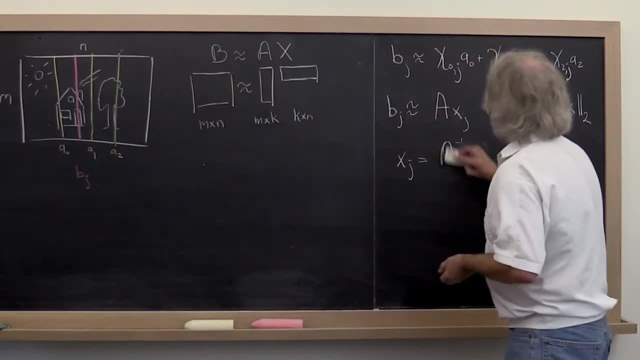 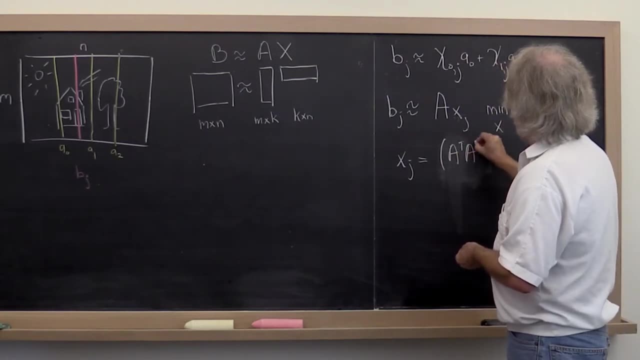 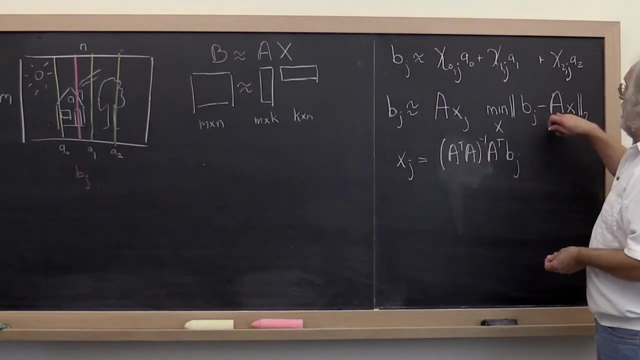 can't do that. Now there's something called the pseudo-inverse that takes its place, And the pseudo-inverse is given by: A transpose A inverse. A transpose times B, j, And you can prove that this is the best choice in the case where A has linearly. 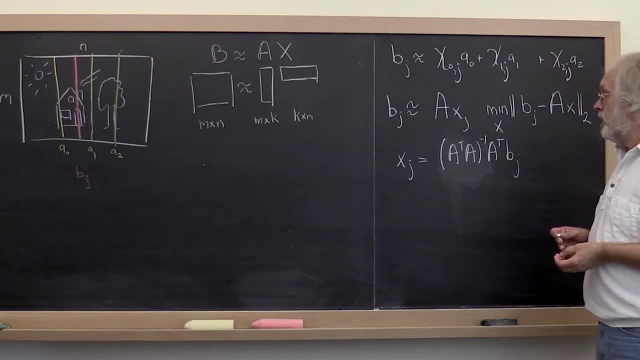 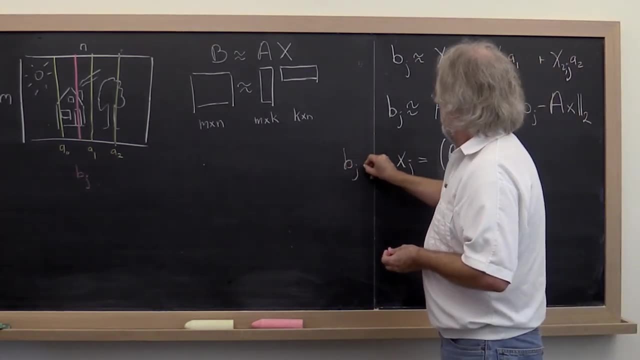 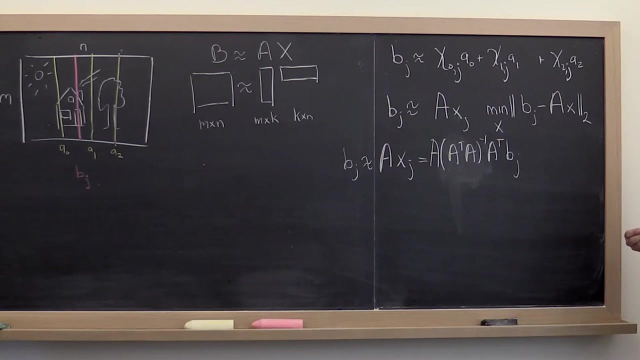 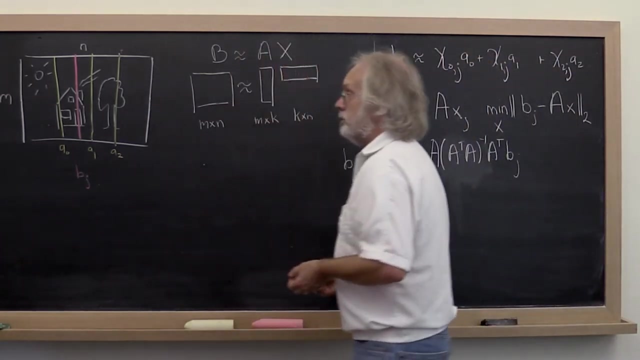 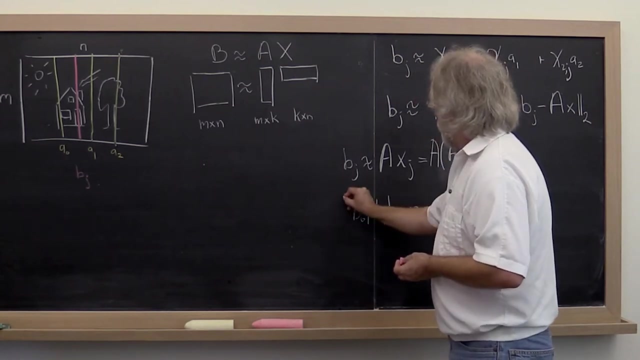 independent columns, right? And what does that mean? Well, that means that our B j is approximately A times that vector which is given by that right there. Now what if we do that for all of our columns in our picture? Then we would say: okay, B 0,, B 1, and so forth is approximately equal to: let's see. 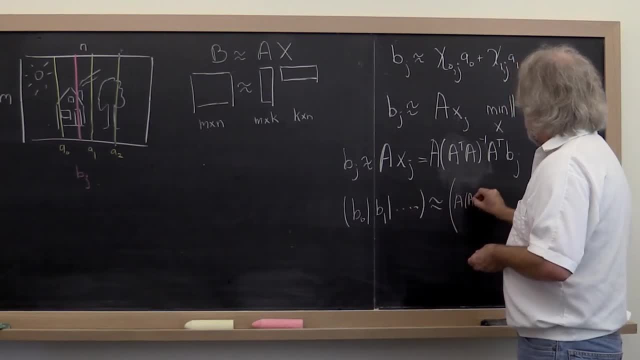 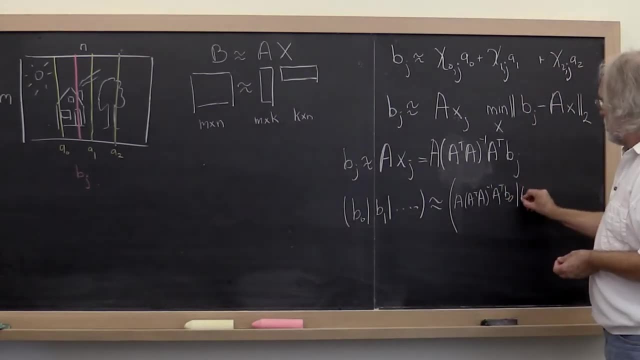 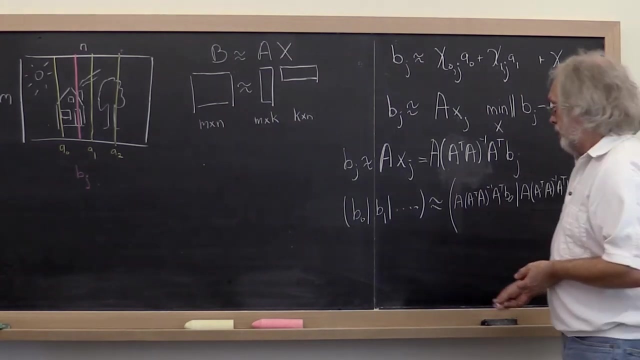 the first column would be approximated by A- A transpose A- inverse A transpose B 0.. The second column would be approximated by A times A transpose A- inverse A transpose B 1, and so forth. And we should recognize the fact that we can then bring this matrix out And this is: 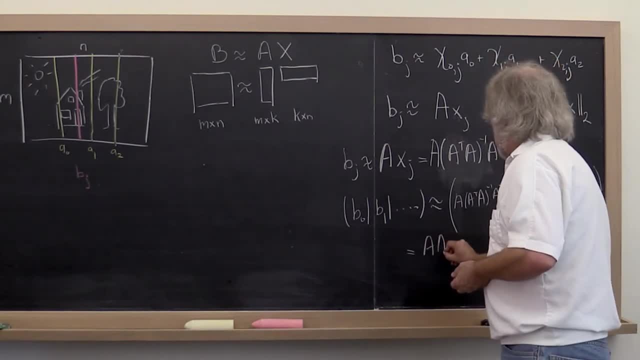 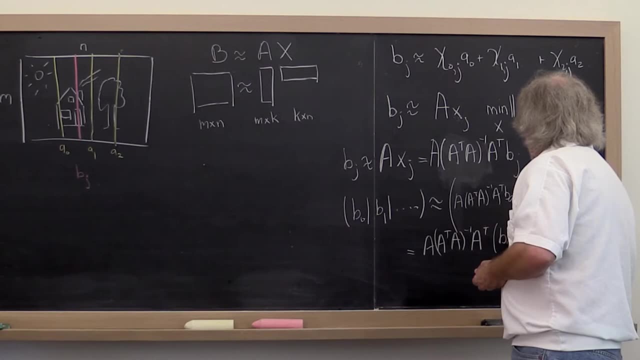 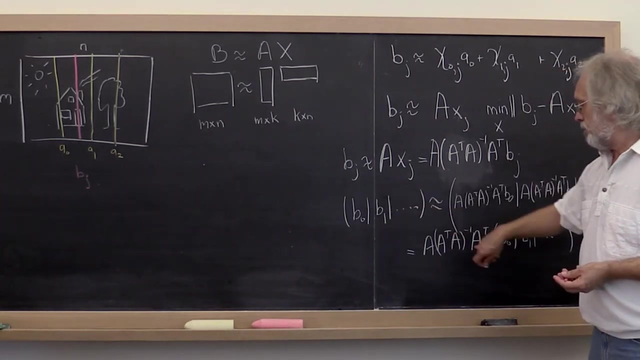 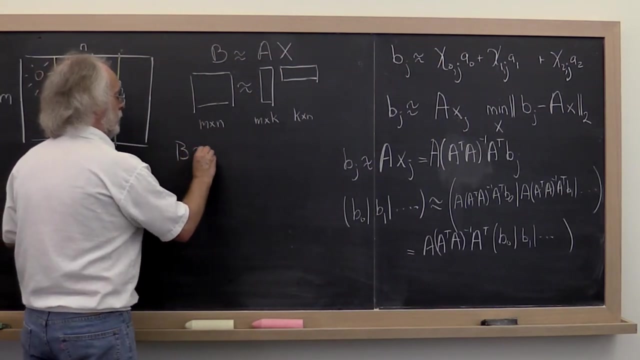 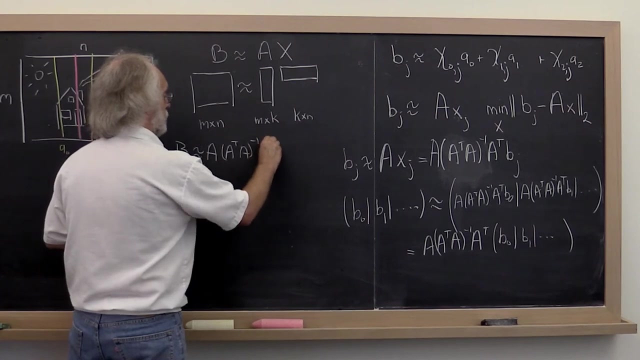 actually equal to A times A. transpose A inverse A. transpose times B 0, B 1, and so forth. This is equal to that and therefore this is approximately equal to that. So what do we have now? We have that B is approximately equal to A times A. transpose A inverse A. transpose times B. 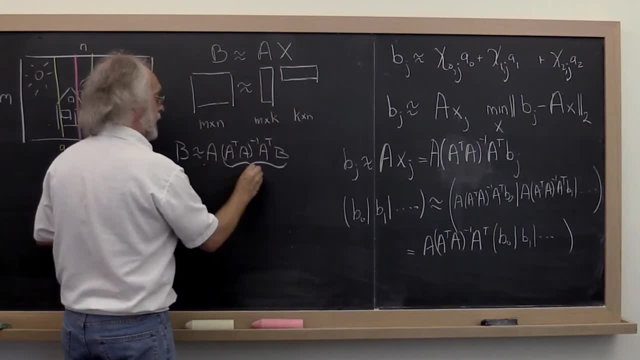 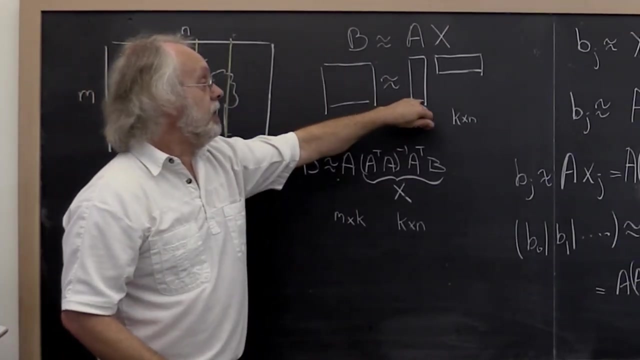 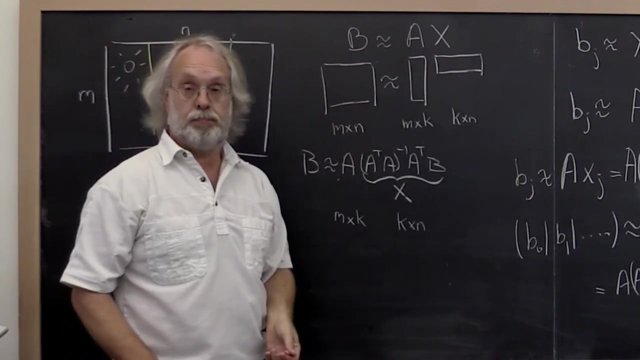 We can choose this to be our matrix X. This matrix is then m by k. in general, This matrix you can check, is k by n, And what we have now is a formula for computing a rank k approximation to our picture. You can check that this is a rank k matrix. All right, Now you can say: well, it. 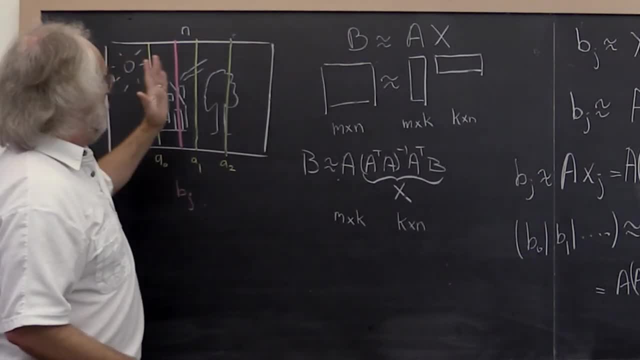 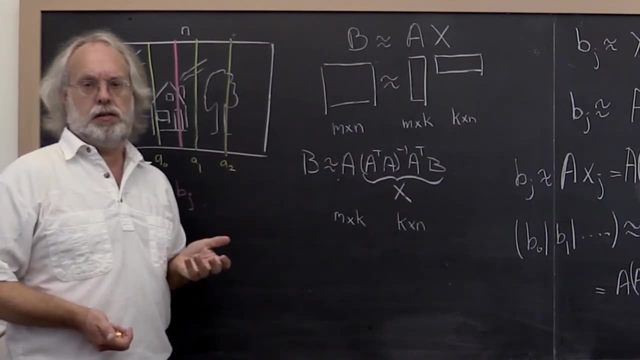 would seem to me that there must be optimal columns in my picture that I can pick to get the best approximation. And then you might say: well, it would seem like a branch of all of these items. is aибin equal toライ, the EmpressESERRORSWOLE, it might seem like a.